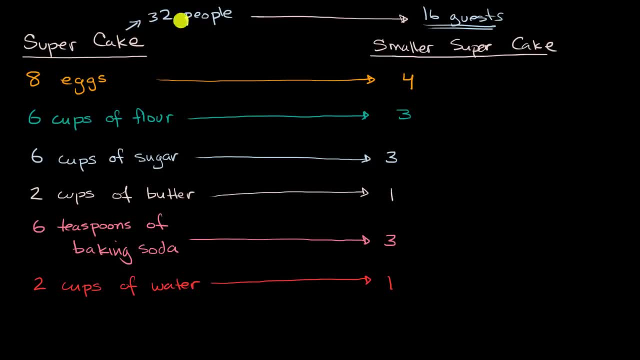 the recipe for the main super cake that feeds 32 people and the recipe for the smaller super cake. And that's the notion of ratios, the ratios between ingredients or the ratio of how much of an ingredient you need for a given guest. So for example, you can see here: 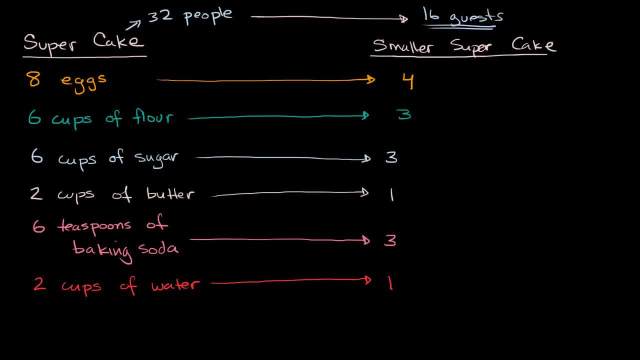 that for every eight eggs you have six cups of flour. So let me write this down. So for every eight eggs we have six cups of flour. We have six cups of flour, which can be expressed as a ratio of the ratio of eggs to flour is eight to six. 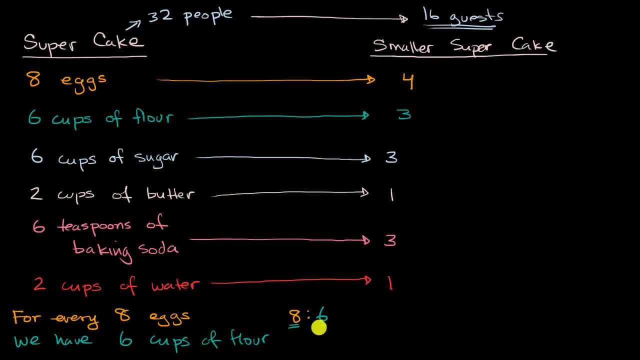 which is once again interpreted as for every eight eggs I have six cups of flour. If I said for every six cups of flour I have eight eggs, I would have written six to eight. So the order here matters. But here I'm saying the ratio of eggs to flour. 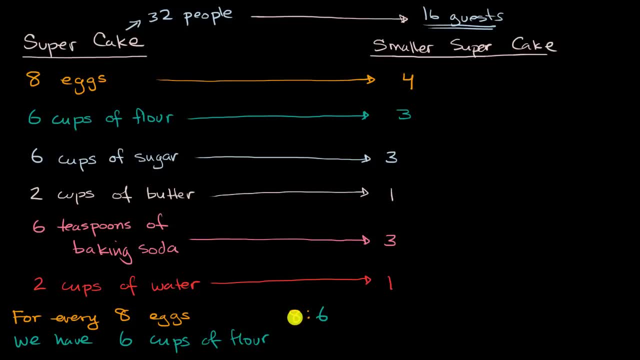 of eggs to cups of flour is eight to six. For every eight eggs, I have six cups of flour. Well, what about for the smaller cake? Well, here, for every four eggs, for every four eggs, we have three cups of flour. 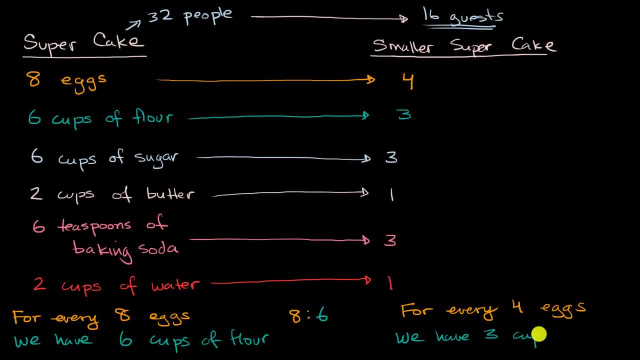 We have three cups of flour. So what would this ratio be? Well, for every four eggs, we have three cups of flour. So the ratio of eggs to flour is four to three. Now it turns out that these are the exact same ratio. 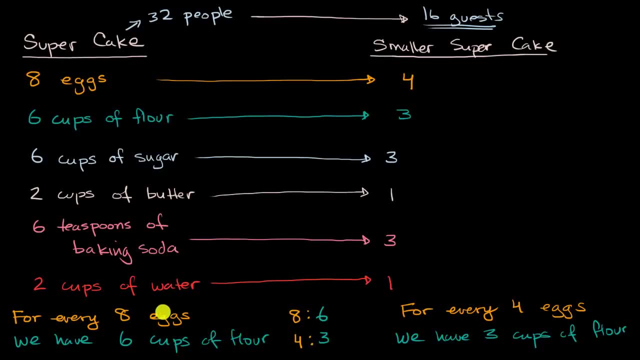 If you have eight eggs, for every six cups of flour, or for every eight eggs, you have six cups of flour. that's the same thing as for every four eggs, you have three cups of flour. What you're just doing is taking each of these numbers. 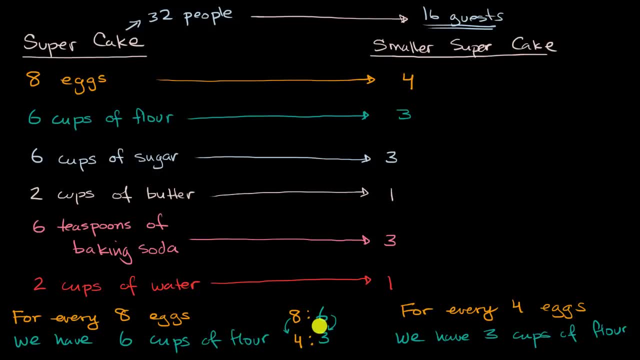 and you are dividing it by two. So you could say the ratio, in either case, the ratio of eggs to flour. let me write this down: the ratio of eggs to cups of flour. let me write this down. let me write it: two cups of flour.